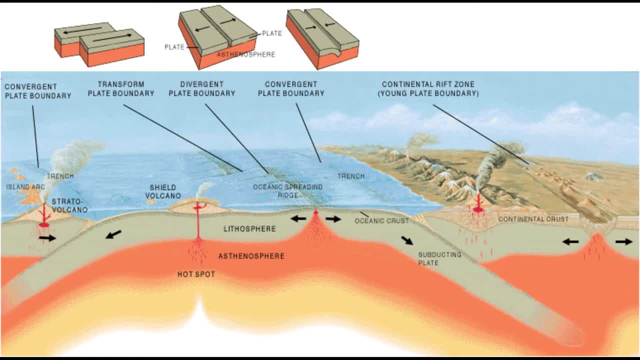 the geological process of mountain building. It's called orogeny. It's result of collision between plates. It involves thickening, uplift and displacement of the crust, with igneous activity folding and folding creating long scars over Earth's surface. So, before the plate tectonics come in place and we 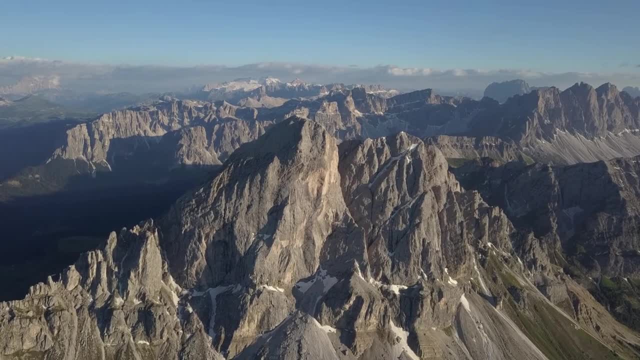 have more clear understanding how mountains are built. geologists only understood that the mountains are growing And it's happening for several or even tens of millions of years. This process can be going on and on and on, But the geologists keep telling us that the mountains are only growing and developing and the mountains are not just a series of mountains. They are not just a series of mountains. 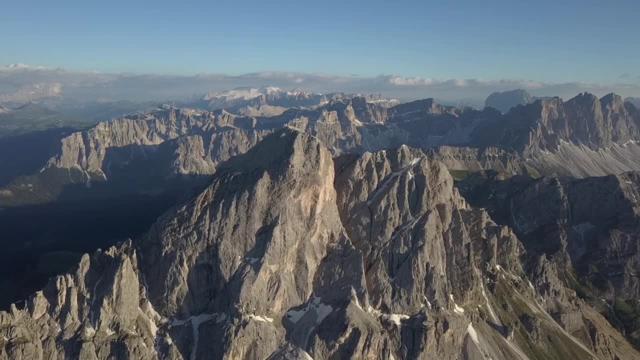 The geologists keep telling us that the mountains are growing with the top. A series of mountains- they are not just the layers that are all raised into one mass- can stop and erosion, the removal of material due to the weather, river streams, snow and so on, making 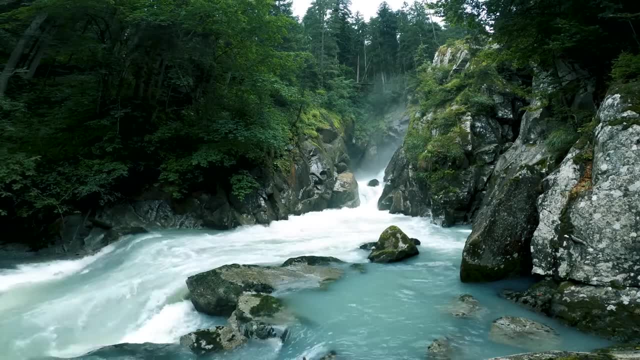 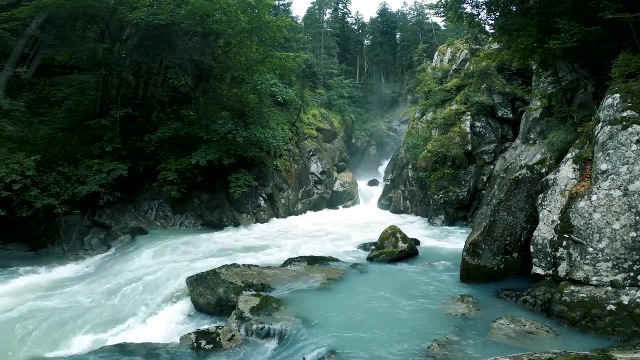 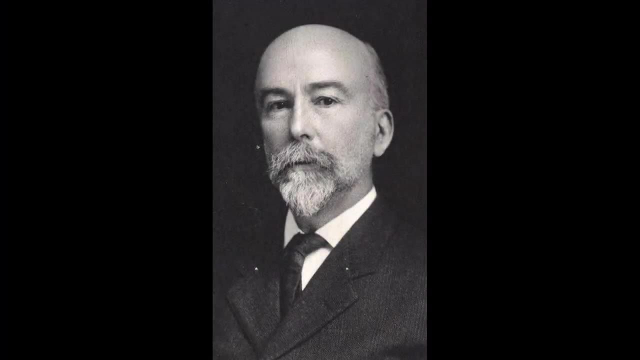 the mountains shorter, kind of flattening them down. therefore, all the rocks which composed mountains of they've been removed down into the ocean back again, where it's come from. however, in 1899 the famous geologist william maurice davis developed a beautifully simple life history of mountains. 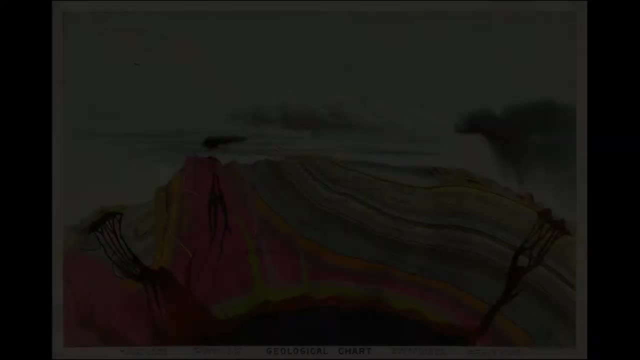 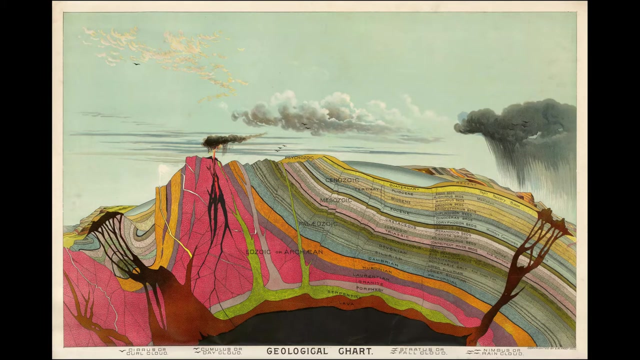 we call it cycle of erosion. he suggested that mountains created in a brief and violent spasm, uplift in the landscape, then a gradual decline through youth, maturity and old age by the forces of erosion which i already talked about. once these mountains become flat again and level with the 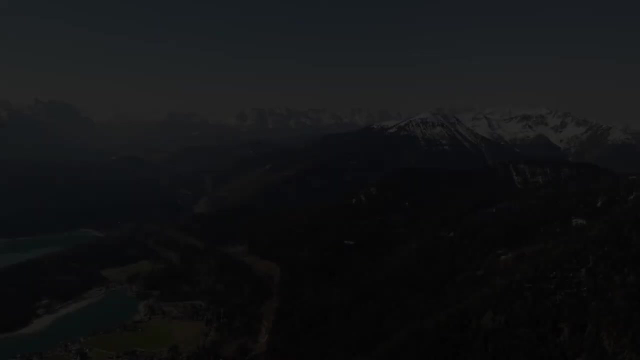 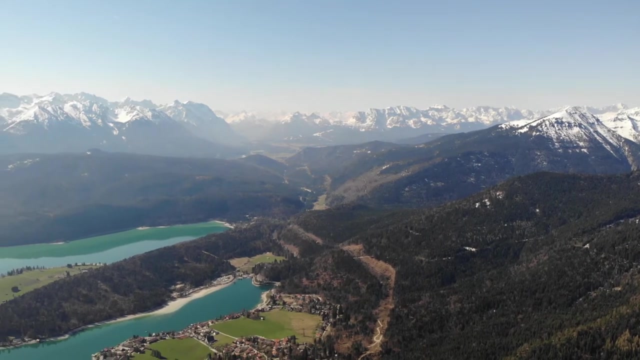 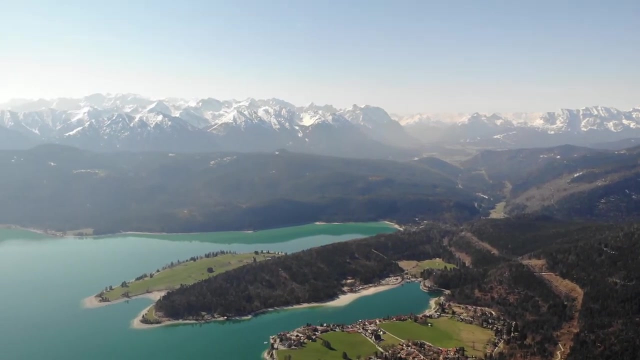 other land around it. another spasm of uplift started the cycle again. of course we understand now that this is not very true. his idea was why the mountains were built in different ways. it was widely accepted. it was the most reasonable and elegant model for that time. it was kind of used by scientists till the plate tectonics developed in. 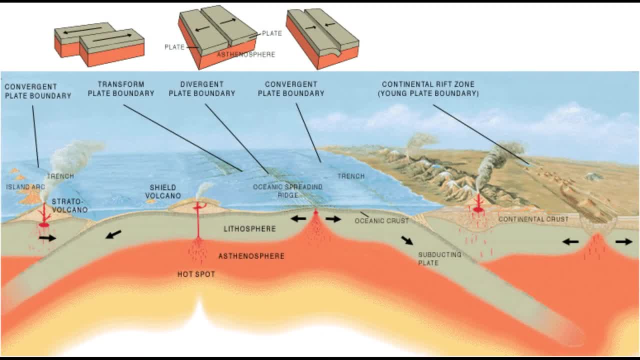 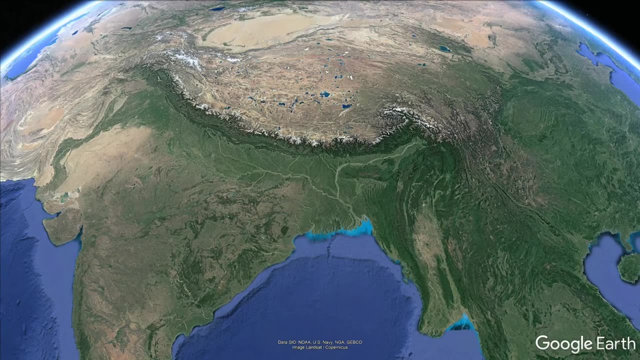 1960s. now we know there's a little bit more behind that. therefore, in modern days, we understand the mountains can be built in different ways. the most ranges we have on our planet these days are built from the collision of two plates. it could be two continental plates, like in case of eurasia, and 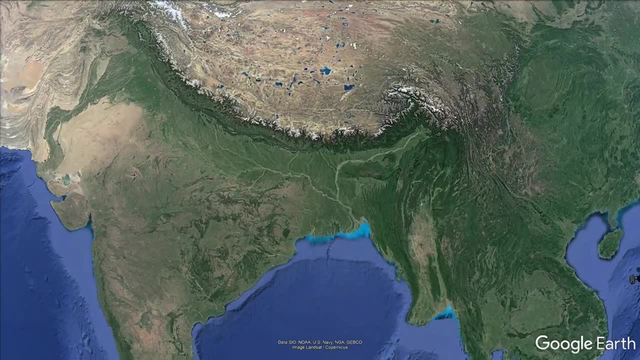 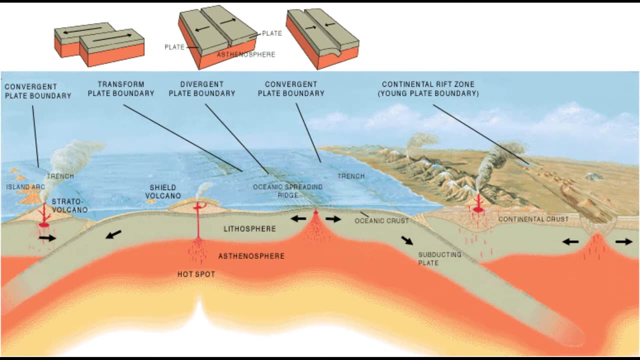 huge himalayas. or it could be collision of oceanic plate sliding under the continental lighter but yet thicker plate, for example undies. all the west coast of america's is north and south, but saying this, remember that on the bottom of the ocean we have mountain ridges as well. 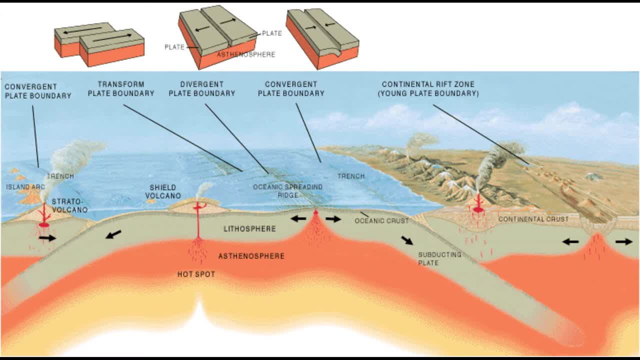 and the famous mid-oceanic ridges. they're formed actually by spreading the plates, two ocean plates spreading apart and this depression start filling with the basalt and the oceanic plates start to rise and the mountains are formed with some volcanic activity. see my video about plate. 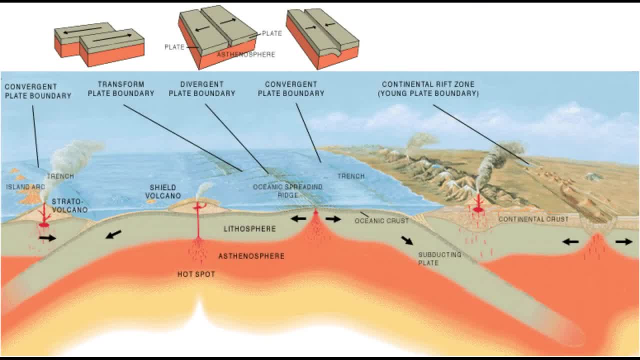 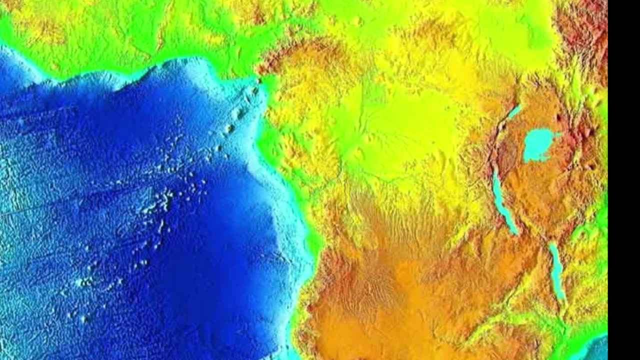 tectonics for more examples and information about that similar. we have places on the continents- we call them rift zones- when in the past one plate start divided and the new ocean crust, future ocean plate start building, for example, eastern part of africa or big rift zone in siberia, where 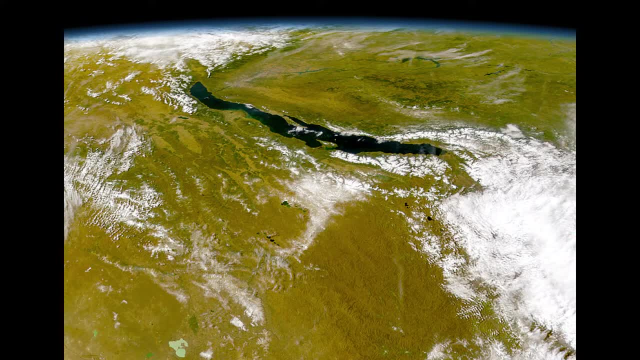 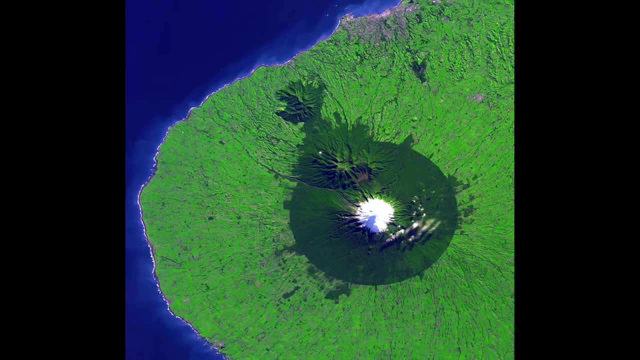 the baikal lake, the biggest freshwater lake in the world, is located in the middle of the ocean reservoir on our planet is filling this depression of two plates. moving apart, you also know mountains which build through the volcanic activity. we kind of call them places of hot spots, for example big volcano or fujiyama in japan. or we have single mountain peaks of large. 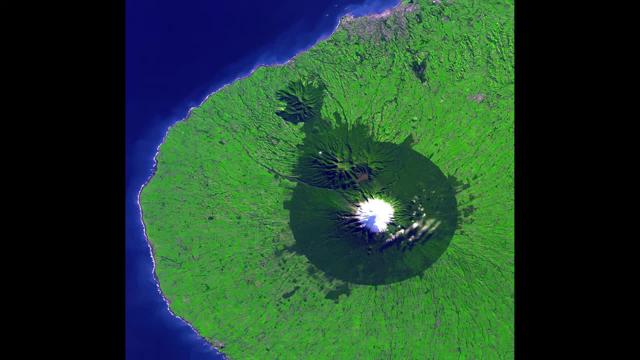 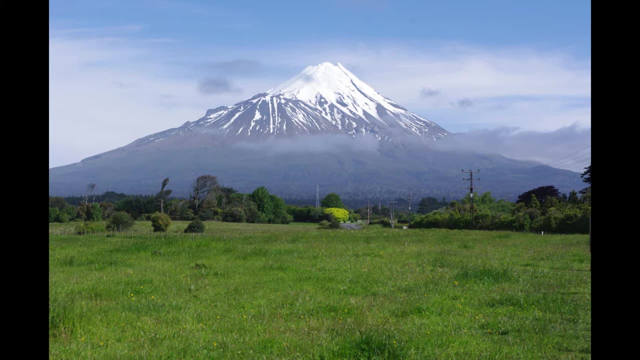 volcanoes like taranaki in new zealand. it seems like they're just standing in a very flat area, nothing around them. but we understand that the hot spot, the warm magma coming closer towards the subsurface exists, rather that moon at. warm heats meet with the sun, so these Humans become rather. 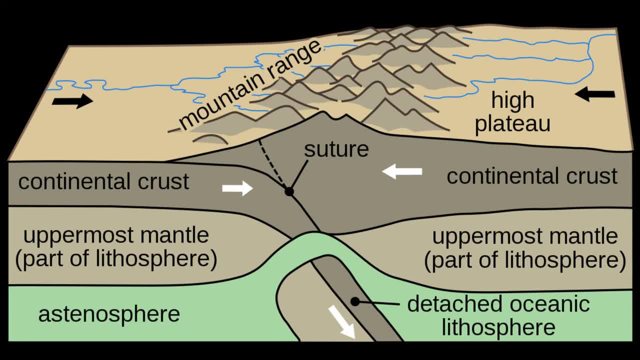 warm täni sfer and it's caused the creation of the volcano. however, all the highest ranges of the land, like you, where two plates are moving together- some i say it's like a rug rumpled against the wall- converging plates- crumple the rocks in. 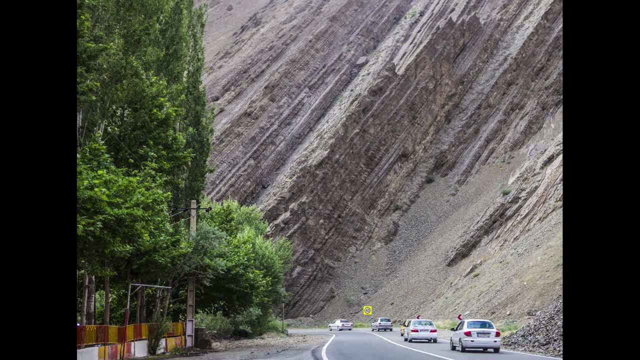 between forcing them to upwards and creating long folds all along the boundary. if you ever go to the mountains and you see some nice exposure, usually along the road- so when you're driving, look at the and you will see this nice folding features which look like somebody put them there. This is all the. 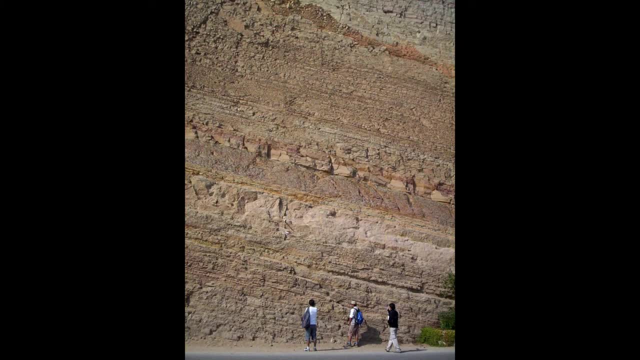 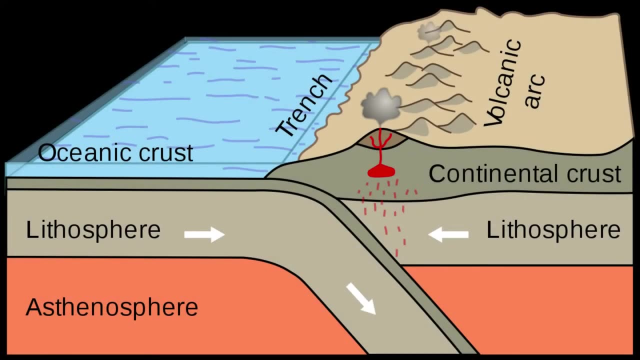 forces of this crumble and folding the layers of the rock one over the other, while the, for example, oceanic crust coming under the continental crust and it starts folding this lighter and yet more viscous layers of continental crust surface As the oceanic play goes on pushing under the continent. 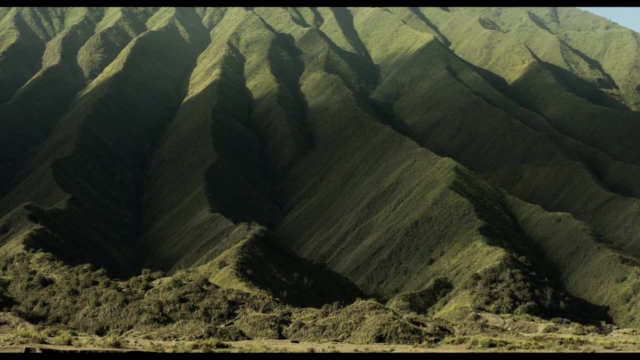 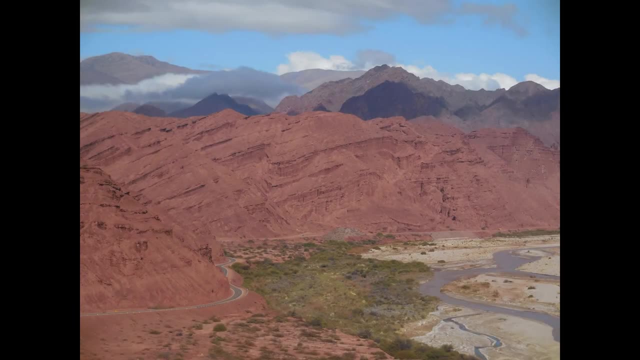 these terrains pile up higher and higher in fractured and folded mountain belts. Think about North American Cordillera, which formed like that. Eventually, when this oceanic crust move towards the continental crust, it becomes consumed by the mantle and it's leaving the continent going towards the continent. This is one of the most violent collisions which we observe on our 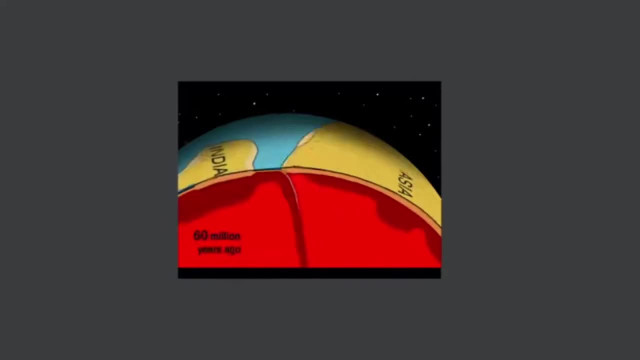 planet- and Himalayas is a great example of that- Two softer and lighter continental plates pushing against each other, and both of the surface materials start been folding against each other. It's a little bit tricky for geologists to understand the landscape there and the map. 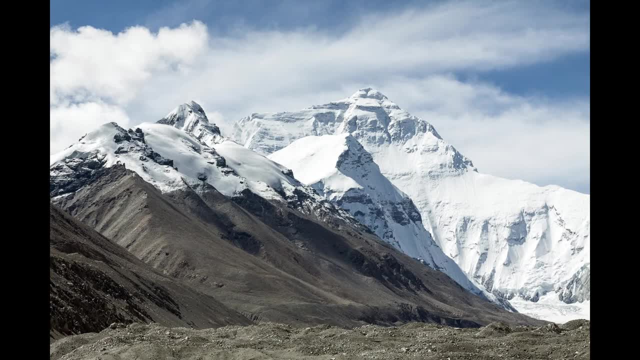 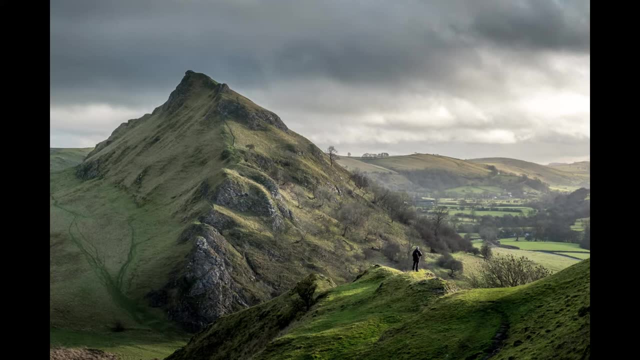 geological feature. You have to do a lot of investigation. However, some mountains built in the past and now they're just left alone. They're not uplifting anymore because continental plates, oceanic plates, change the direction of movement and they slowly start reducing the height. so they're not. 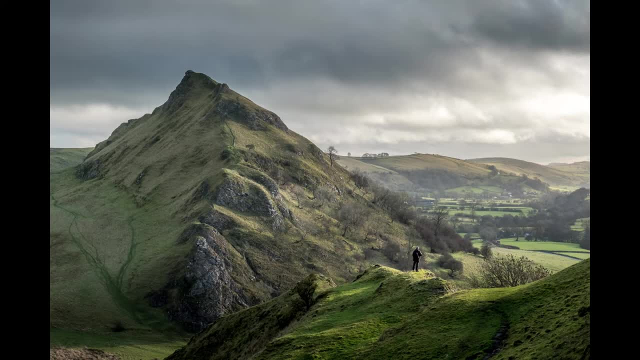 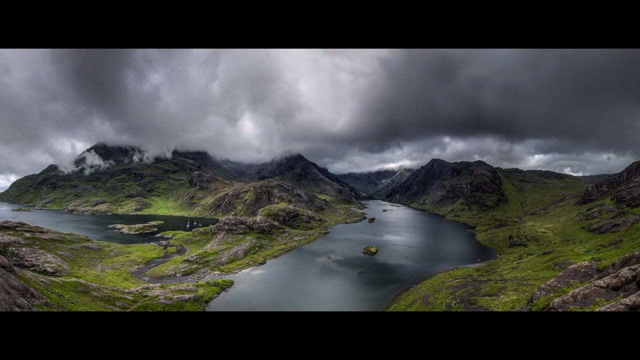 uplifting- They're not active anymore- and erosion, removing the material helping to flatten them down. You know some of the mountain ranges, such as Appalachian mountains in North America. they used to be formed when Africa and North America collide. Similar in Scotland and Norway we have Caledonian mountains, which formed in the same way back in the past, before even continents. 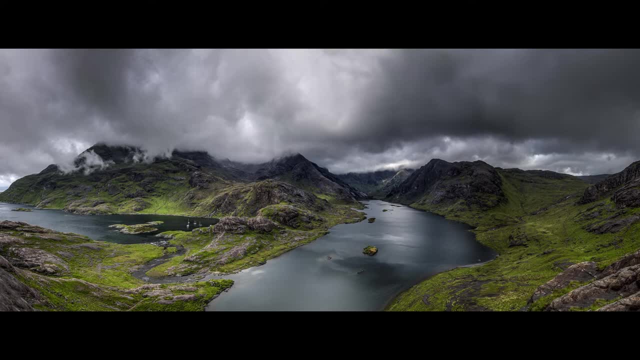 were, as we know them now, Europe and North America. that time collide towards each other Right now. if you visited Scotland or remember the landscape of Scotland, it's very rolled landscape with not such a tall mountains and unfortunately they only become lower with time. But what about? 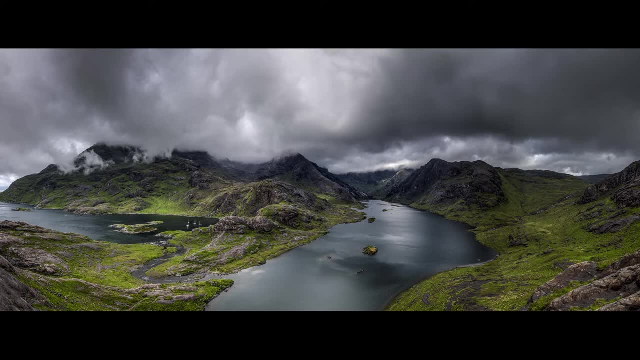 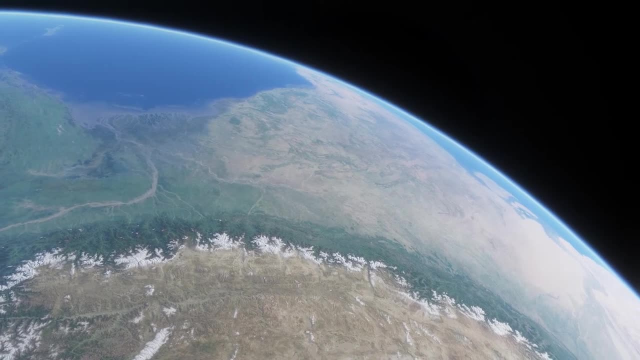 the erosion. There's an interesting relationship. For example, some mountains like Himalayan when they start building up and creating this huge Tibetan Plateau with the highest mountains all around it. You know, in the northern part of the Tibetan Plateau you can see the northern part of the. 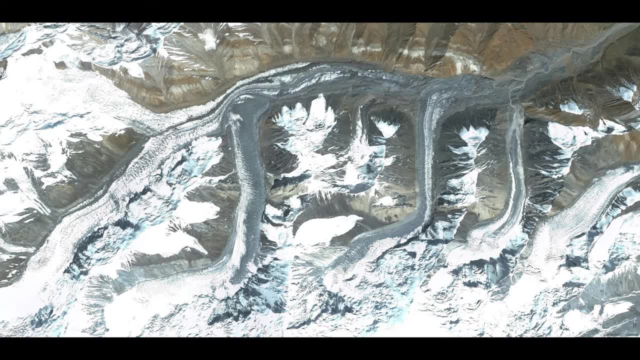 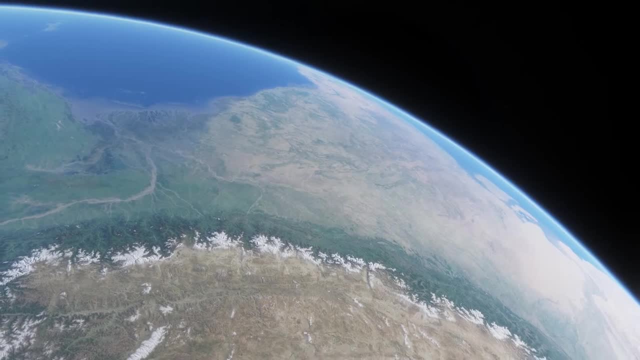 We have 7,000 peaks in the countries like Kyrgyzstan, Tajikistan, China. All the southern mountains are the highest peaks we can find on our planet. right now, This huge plateau. when it starts forming, it changes the local climate in that area. 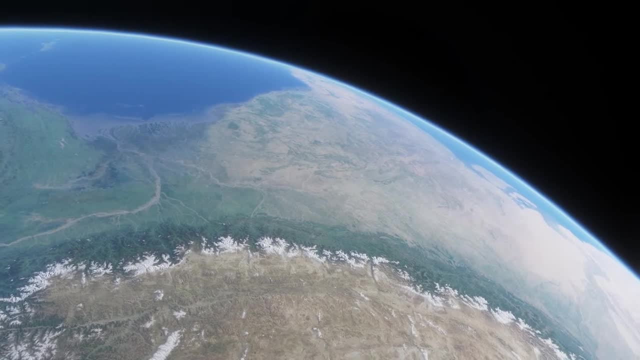 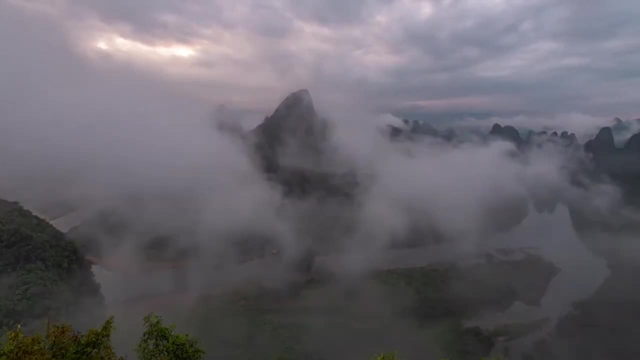 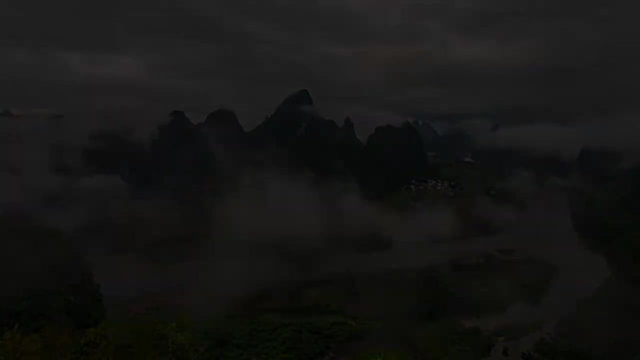 and the monsoon starts affecting these mountains and whole India and other countries around it. As a result, huge amount of water starts falling down seasonally in that area and the erosion dramatically increases. We have constant uplifting of the mountains because one plate going towards the other. 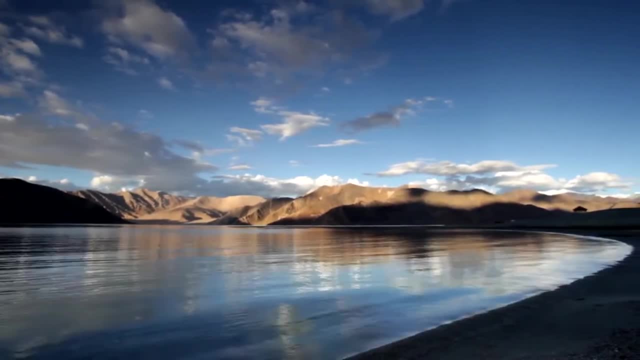 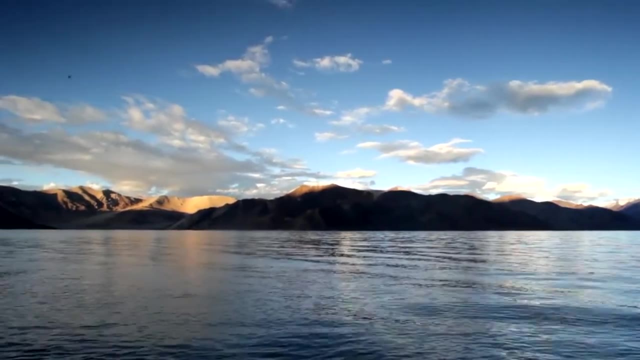 with a high speed and at the same time, we have very, very high erosion rates, reducing its height. But even though we have such high rates of erosion, the mountains are still uplifting and scientists suggested about 5 mm of Himalaya every year growing higher up. Therefore, if you come to Kyrgyzstan, you will see that the mountains are still uplifting and the mountains are still uplifting. Therefore, if you come to Kyrgyzstan, you will see that the mountains are still uplifting and the mountains are still uplifting. 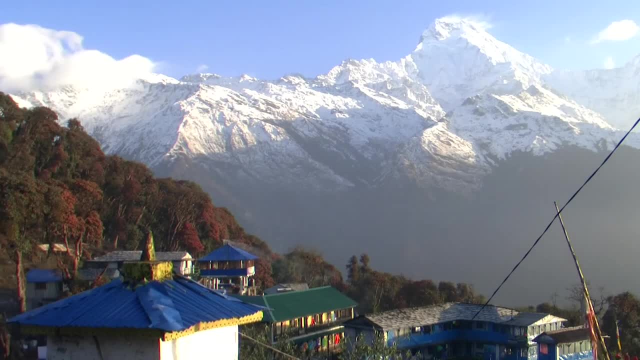 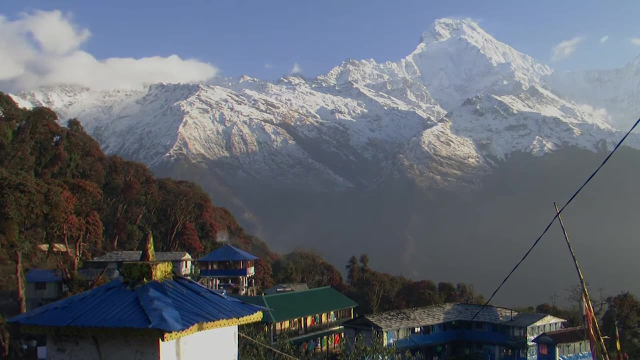 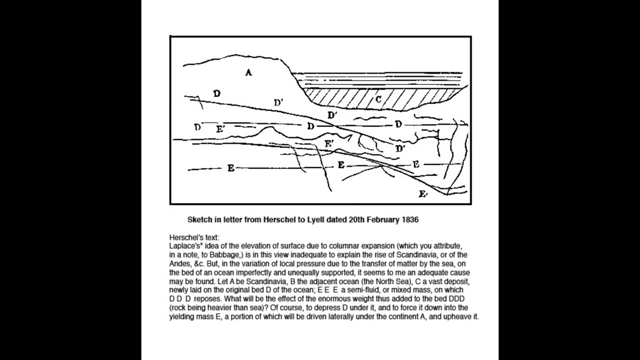 If you come back in 10 years to Himalaya and wanting to climb the highest peaks there, you will beat the previous records. Erosion also can invoke asostasy. This is when the mountains, which used to be heavier. they are a little bit kind of. 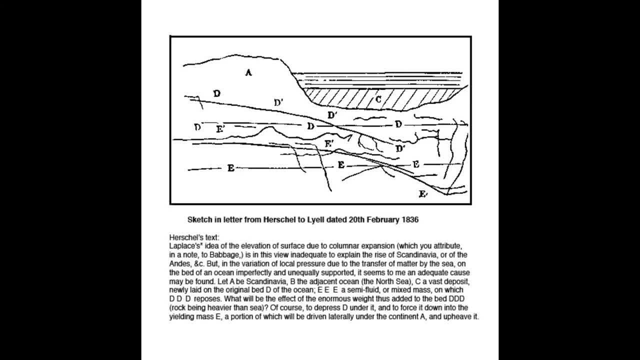 like beyond, on the mantle, on our Earth, and they were a little bit sunk deeper, with the roots going deeper into the highest levels of asthenosphere. When you start removing material from top, the crust becomes lighter. When you start removing material from top, the crust becomes lighter. 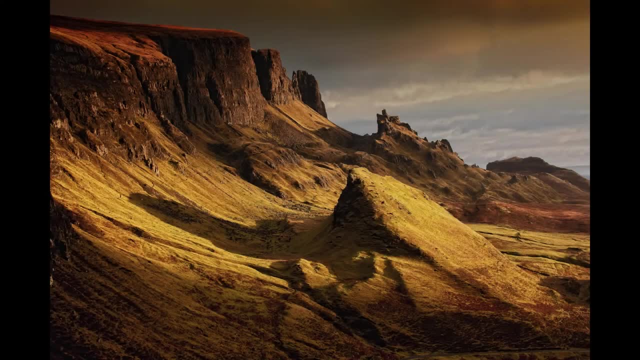 And start a little bit uplifting because of asostasy, not because the mountains are uplifting by pushing plates. So when you are looking on the charts of mountains, the uplifts, you need to calculate that. You need to calculate natural uplift due to the plate, tectonics uplift due to the asostasy. 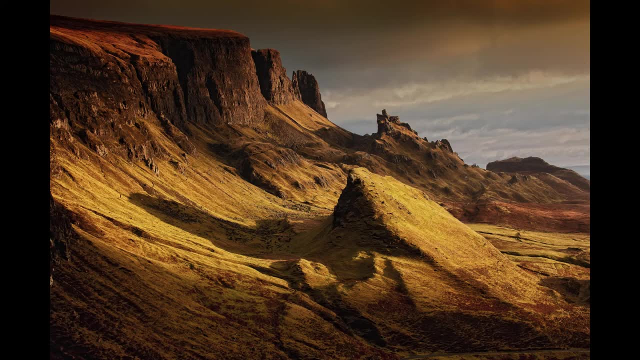 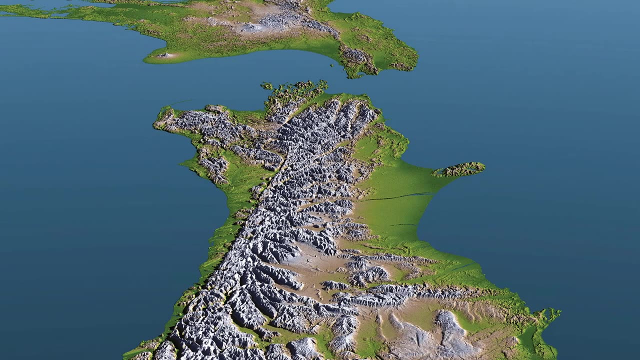 and reduction of the height due to the erosion, An eventual number like 5 mm in Himalaya. it will be that number after all the calculations In the history of New Zealand mountains, Southern Alps- one of the most active places on our planet right now. if there was no erosion, the Southern Alps would be as high as 20 km. 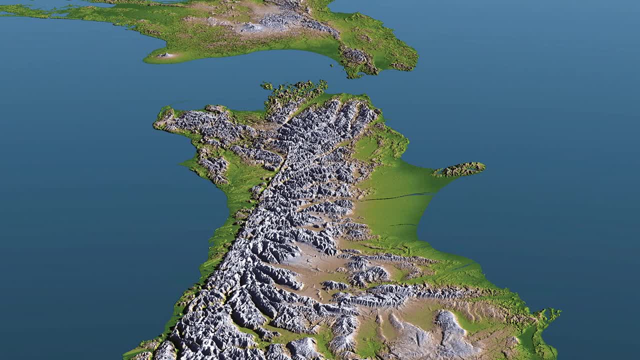 only during the last 2-3 million years of the uplift, That would be as high as 20 km. However, we have very, very high rates of erosion because all this western wind and snow and rain removing the material from it. 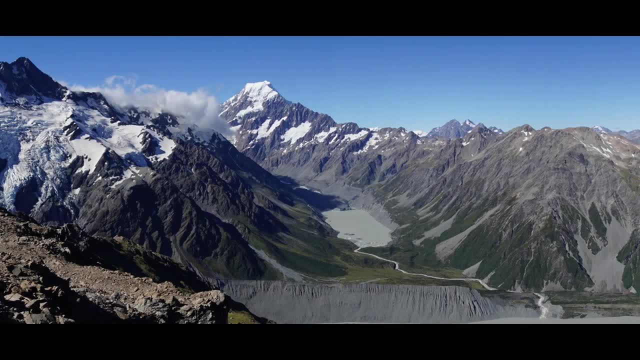 So this means that there would be earthquakes, trigger landslides, slips formation which move a lot of material down through the rivers and we have the mountain peaks not as high.